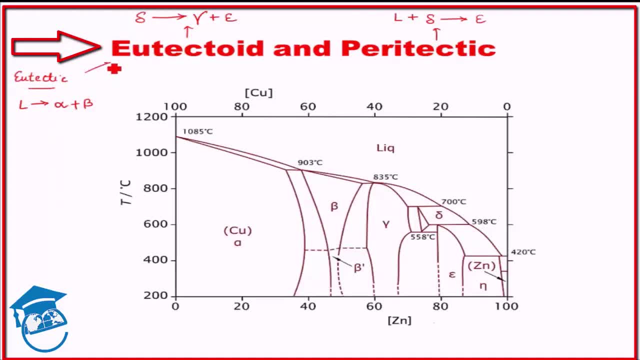 So when we compare eutectic reaction and eutectoid reaction, what we see is that in eutectic reaction, one of the reactant was in the liquid phase, and liquid phase give rise to two different solid phases, Whereas in eutectoid, the reactant is also in the solid phase And similar to 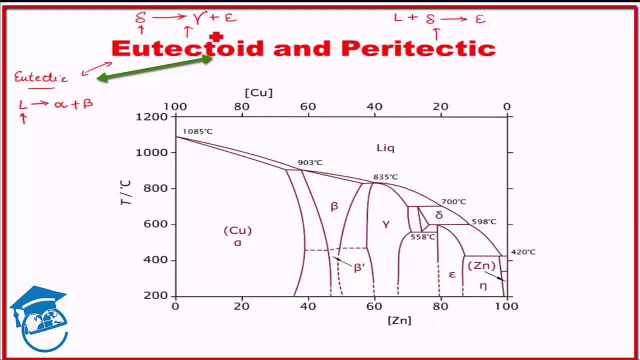 eutectic reaction it is giving rise to two solids. So basically the only difference is: in eutectic the reactant was liquid. in eutectoid the reactant is solid, Whereas in peritectic reaction what we have is a liquid and a solid combines to give a different solid phase altogether. 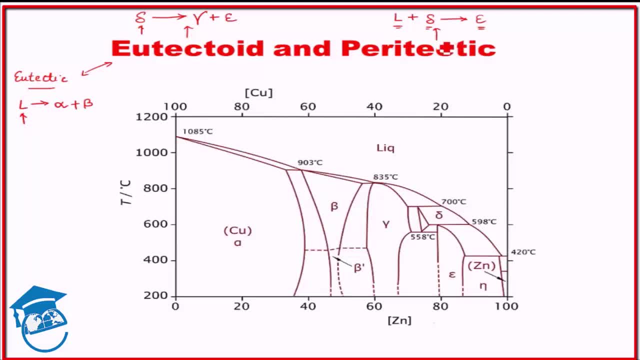 I would like to drive home a point that any reaction, any invariant reaction which has a liquid phase involved in it ends with the tic like eutectic and peritectic. So this shows that one of the components, one of the phases involved is in the liquid phase, Whereas if 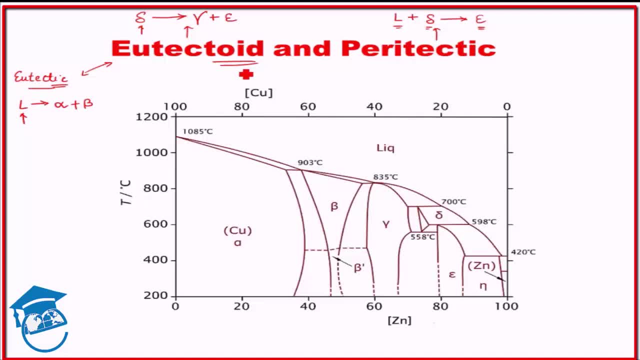 we have toit, the ending as toit. All the reactants are in the solid phase. There is no liquid phase involved. Similarly, we have monotectic, monotectoid. we will not go into the details of those. Okay, now let's see them appearing in the phase diagram. Let's see eutectoid and peritectic. 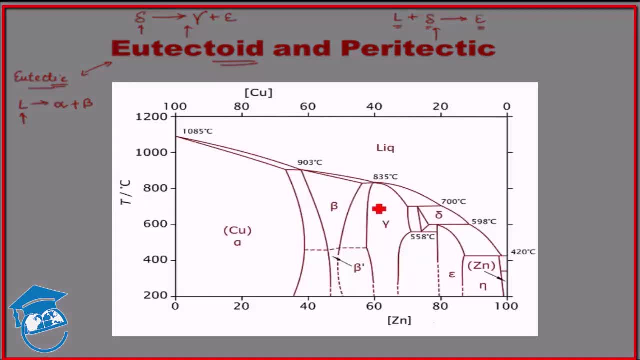 appearing in the phase diagram. So here, as I said, eutectoid is one solid to two solids. This phase over. here is the liquid phase. So here is the delta phase. Okay, this phase is a single phase region and this is the invariant. 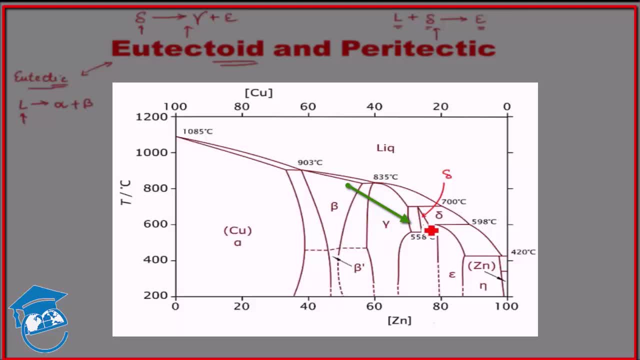 reaction at 558 degrees Celsius. This transformation is the invariant transformation Which is giving rise to gamma and epsilon phase. So this reaction, delta giving rise to delta solid, giving rise to gamma and epsilon phase. So this reaction, delta giving rise to delta solid. 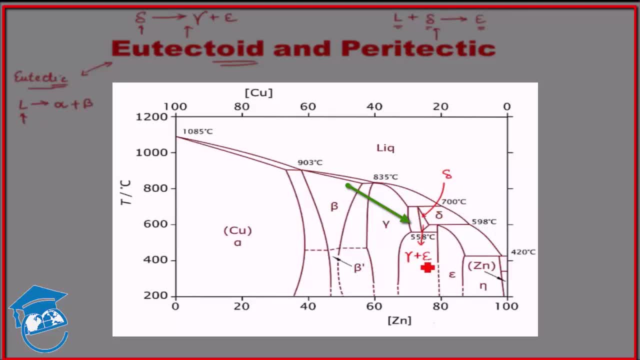 and epsilon solid phases is the eutectoid reaction. We will see that eutectoid reaction also takes place in the iron carbon phase diagram when we study it. I had already mentioned that eutectic reaction takes place in the iron carbon. 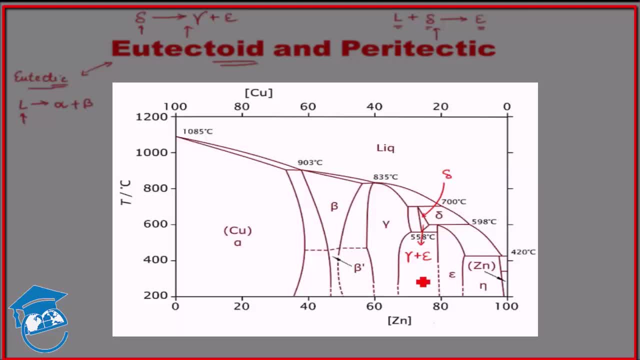 phase diagram. Eutectoid reaction also takes place in the iron carbon phase diagram, Similar to the formation of two solids in the eutectic reaction. the two solids formed in the eutectoid reaction is also lamellar in structure because 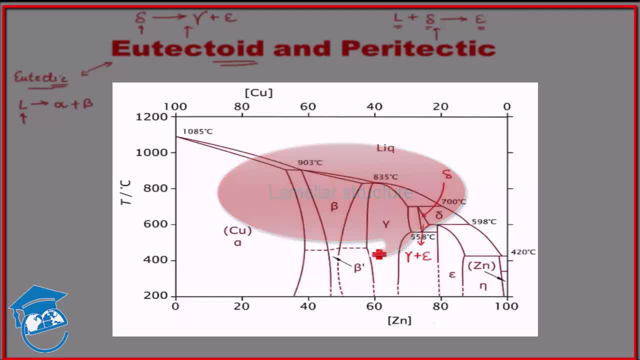 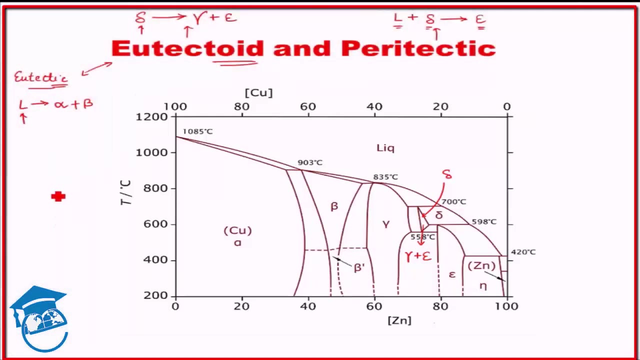 even here, one solid needs to simultaneously give rise to two new solids. Therefore, the grains cannot be independent of each other. They need to be forming simultaneously There by what happens in the eutectic. we had liquid to start with, but in 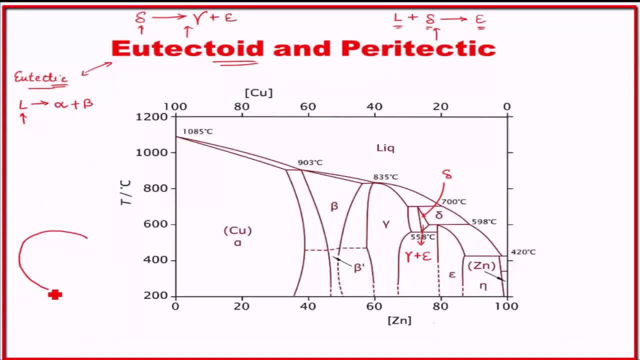 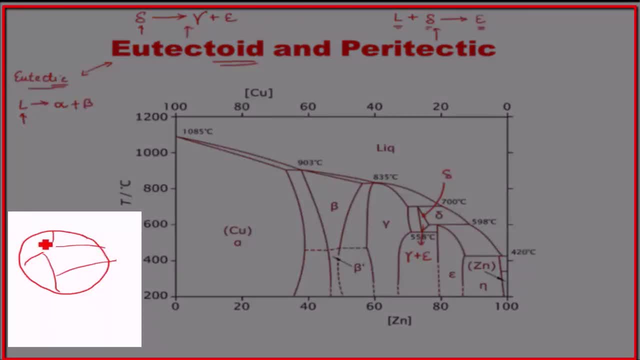 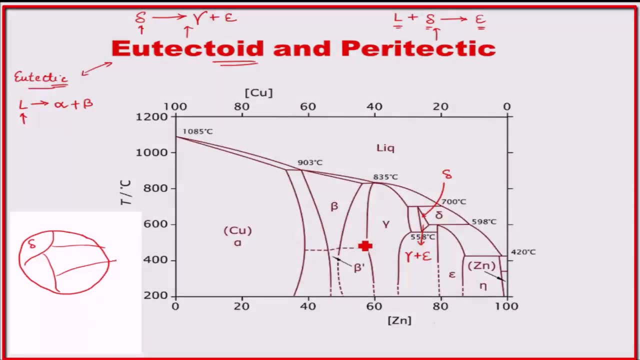 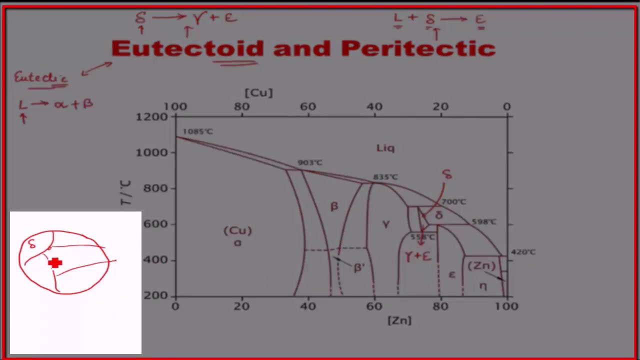 eutectoid, we have solid. so what will happen here is suppose? to begin with, we had delta phase. right, This was delta phase. Once we cool it to eutectoid temperature, what will happen is nucleation will take place at the grain boundary, because grain boundary nucleation is much. 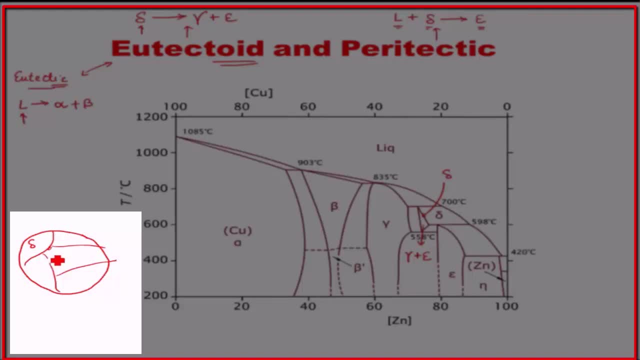 easier, because the energy required for nucleation at grain boundary is lesser than nucleation required for bulk nucleation. So nucleation will take place at the grain boundary, and then the new grains, the gamma and the epsilon grains, will start to grow at the expense of the old delta grains, and they will 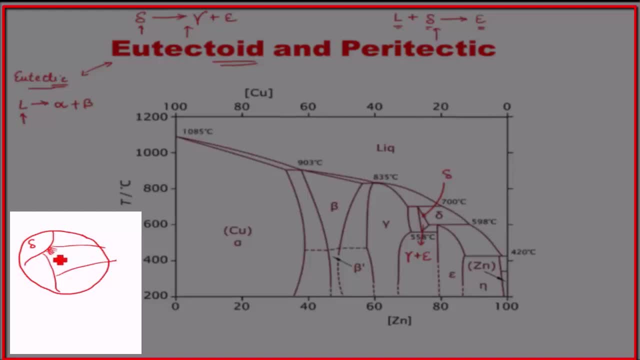 grow in lamellar structure. At the end of the reaction, what will happen is the whole delta. this delta will start to grow. It will be replaced by lamellar gamma and epsilon. like this, The whole. there will be no delta anymore, it will be gamma and epsilon. 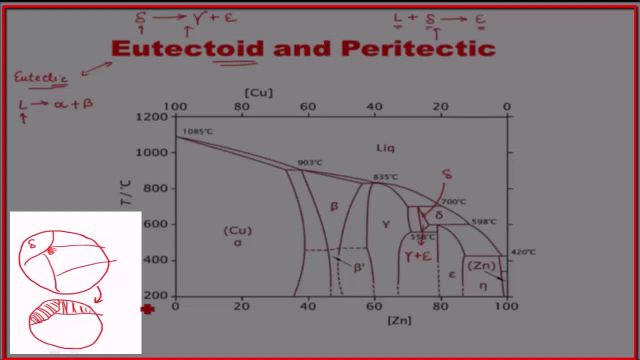 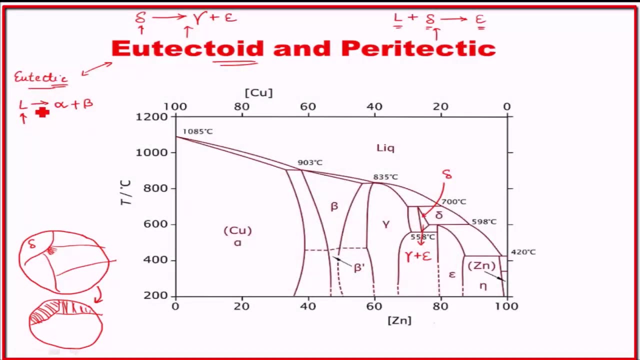 The whole structure will be like that And similar to the case of eutectic reaction, where, even if we did not go exactly at that composition, Even if we were at a different composition, the ultimate, the last bit of solid that will remain in the form of delta will be of the eutectoid composition and the rest delta that 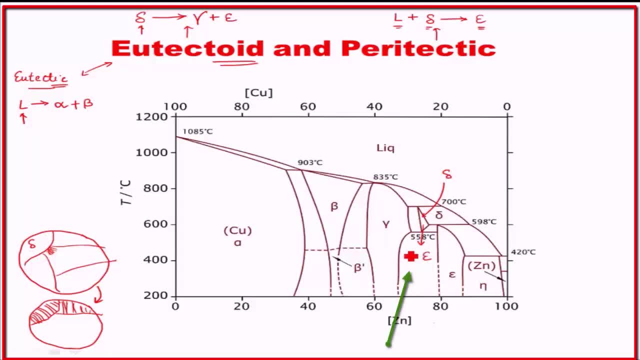 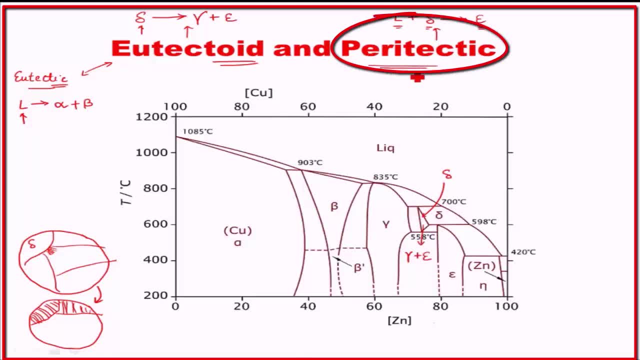 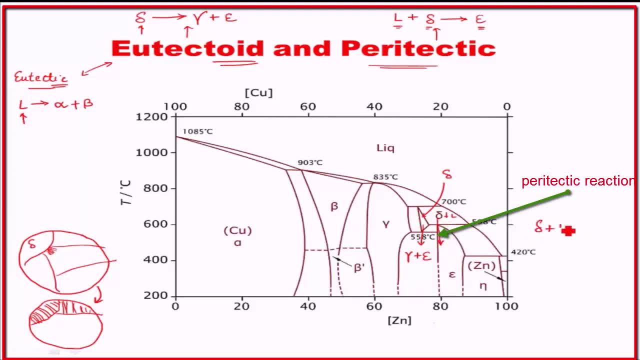 This is the peritactic reaction, where by delta plus liquid gives rise to epsilon. okay, The peritectic reaction also occurs in the iron carbon phase diagram. So all the three invariant reactions which we have studied till now: eutectic, eutectoid. 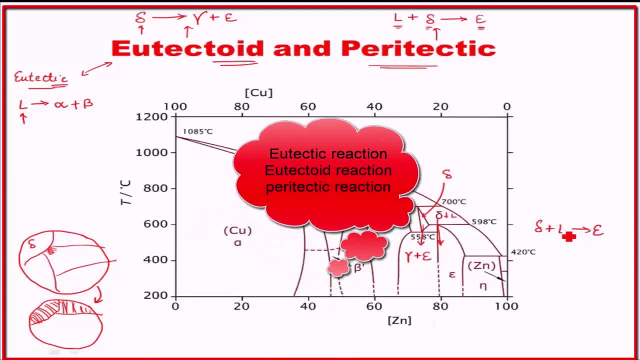 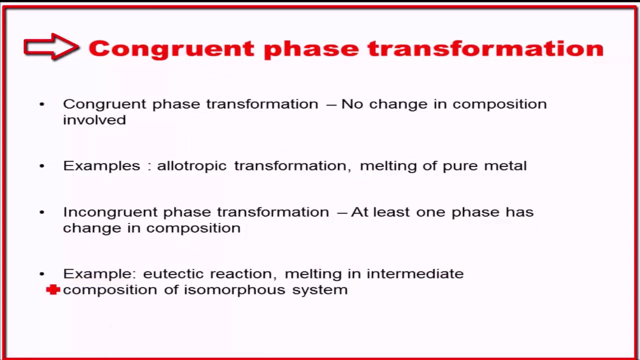 and peritectic reaction. all the three will be occurring in the iron carbon phase diagram. With this, two new invariant reactions introduced to you, let us now jump into some other details about phase diagram and phase transformations. To begin with, let's understand what is congruent phase transformation and what is incongruent. 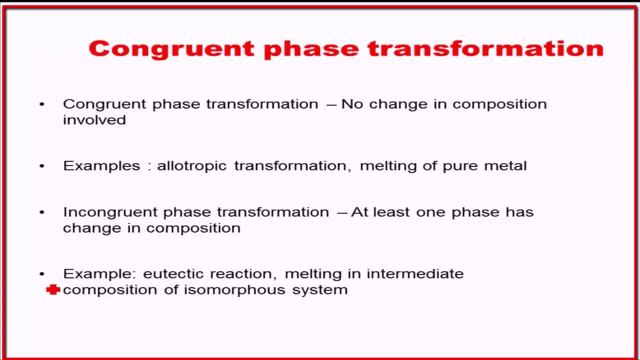 phase transformation. Congruent phase transformation refers to those phase transformation which does not involve any change in composition, So no change in composition involved. Examples of such transformation: Allotropic transformation. Allotropic transformation basically means there are certain elements or certain metals which exist in different allotropic forms. 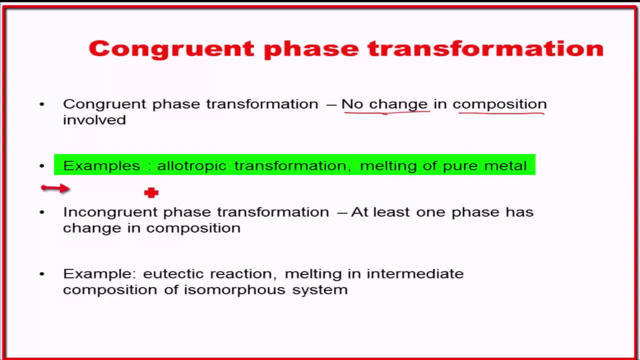 Like iron can exist, as in the alpha form it is body centered cubic, whereas in gamma form it is phase centered cubic. So this transformation of alpha iron to gamma iron, or the other way round, is a congruent phase transformation, Because the composition does not change. 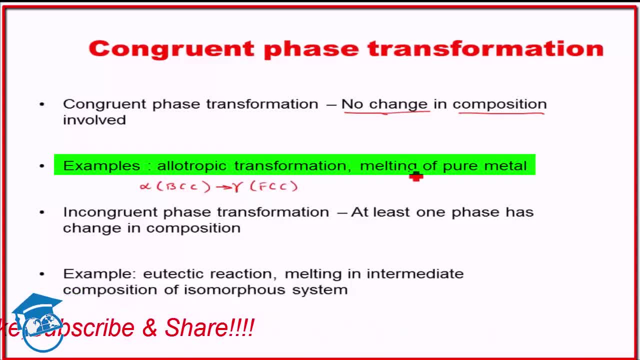 But the phase is changing Again: the melting of a pure metal. Let's say we have a pure iron and we heat it to 1538 degree Celsius. This is solid. We get iron in the liquid form. Iron remains iron. This is 100% iron. 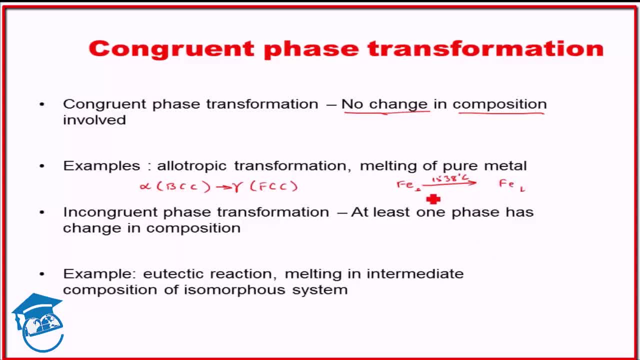 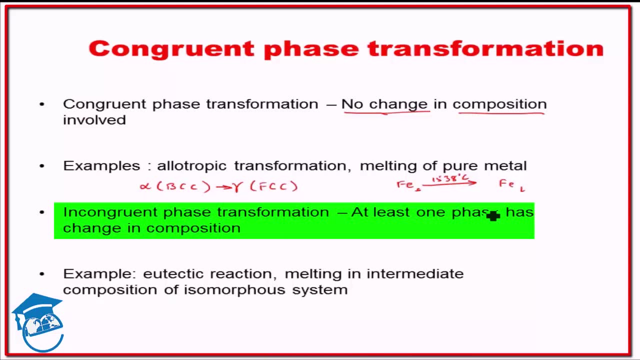 This is 100% iron. There is no change in composition, But there is a change in phase, from the solid to the liquid phase. Therefore, this transformation is also a congruent phase transformation. On the other hand, incongruent phase transformation is one where at least one phase has a change. 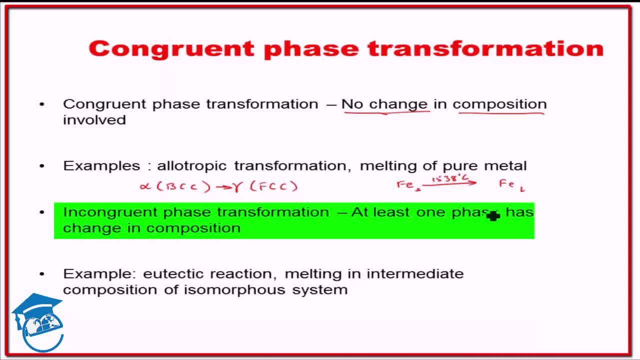 in composition. So if any of the involved phases changes its composition, then we have what is known as incongruent phase transformation. Examples: Almost all the reactions we discussed till now- Eutectic reaction, Eutectoid reaction- All of them have a change in composition. 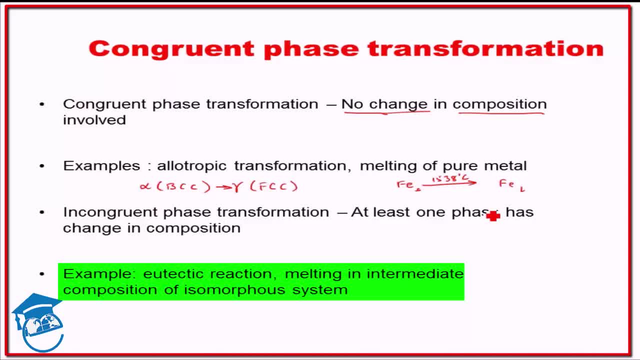 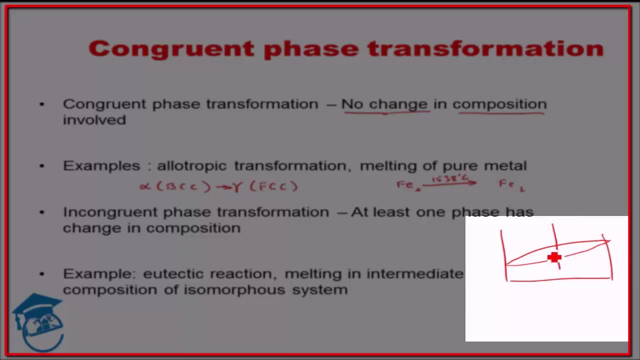 So they belong to congruent phase transformation, Then again melting in intermediate composition in isomorphous system. Like if we have a isomorphous system and melting takes place As soon as it enters the region, the two phases starts having different composition than the. 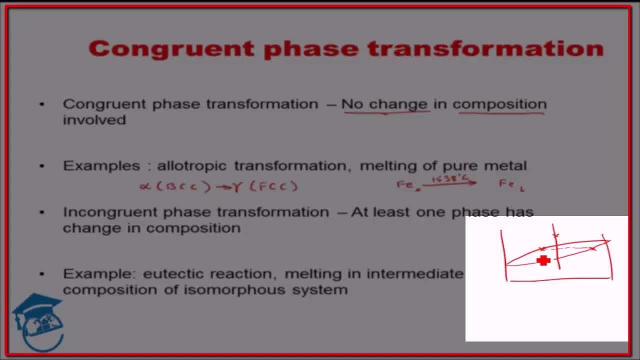 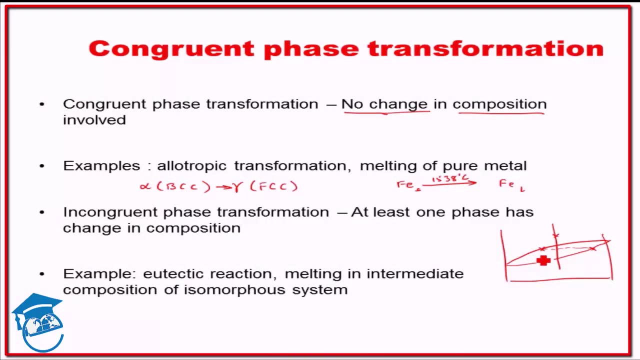 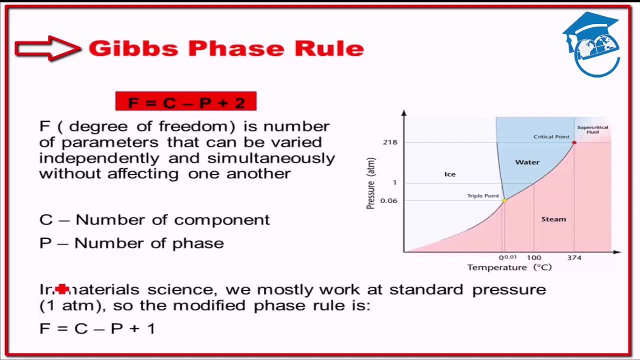 original phase. Therefore, there is a change in composition, Thereby this reaction is also an invariant phase transformation. I hope this makes abundantly clear what is the difference between congruent and incongruent phase transformation. Now, this is one of the important rules I have briefly mentioned about this: Gibbs phase rule. 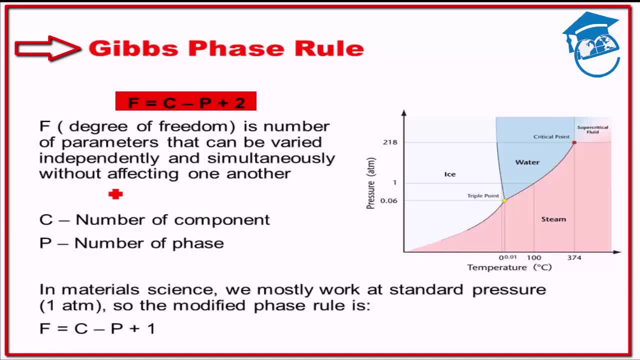 Gibbs phase rule. It tries to relate the degree of freedom that is available and given, C- number of components and P- number of phases. Now what is degree of freedom? Degree of freedom basically refers to the number of parameters that can be varied independently and simultaneously without affecting one another. 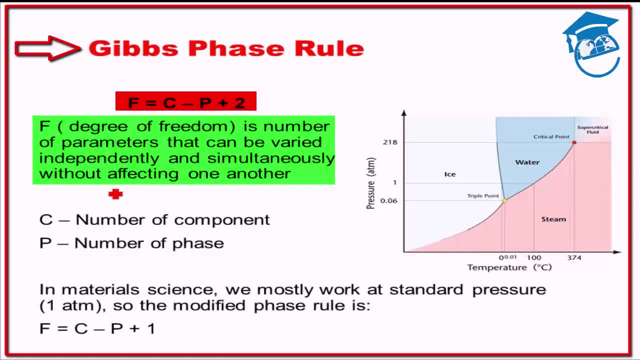 Okay, I will explain you the whole idea of Gibbs phase rule Using The phase diagram for water. But let me state out the rule. What exactly is the rule? The rule is: rule tells that number of degree of freedom is. this is component, C is number. 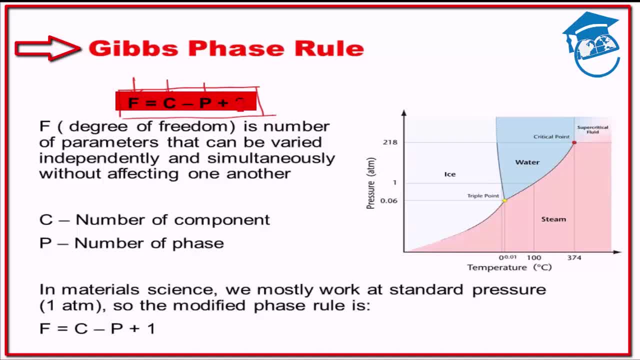 of component, minus number of phases, plus two. You might ask. where does the plus two comes from? the plus two is basically one contribution from temperature, Okay, And another contribution from pressure. So if pressure and temperature can be variables, then we add a plus two over here. 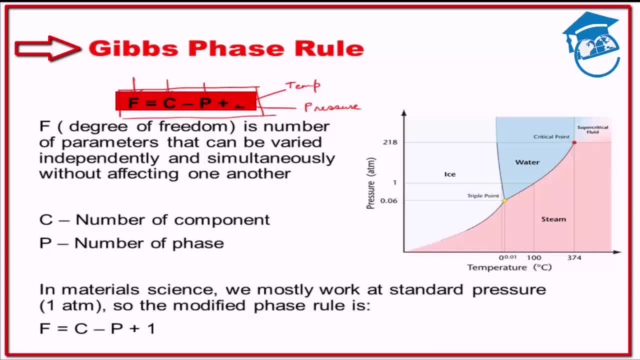 In case of solid state physics, in case of solid state materials, like the things which we will mainly discuss in material science and metallurgy, pressure is mostly constant. We work under standard pressure conditions. So instead of F is equal to C minus P plus two, we take pressure constant and thereby 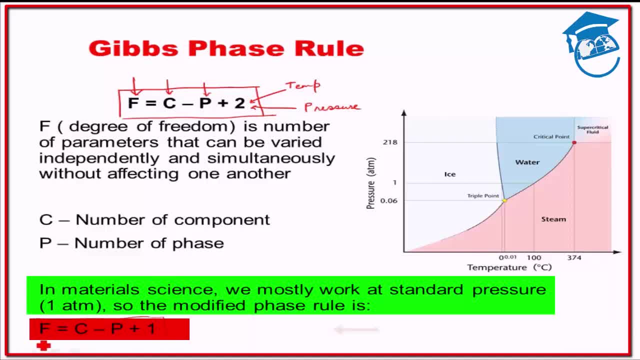 what we get is a modified Gibbs phase rule, which is: F is equal to C minus P plus one. We remove pressure, remove pressure. This is the case in most of the solid phase diagrams which we will study. But now let me explain this with the help of: 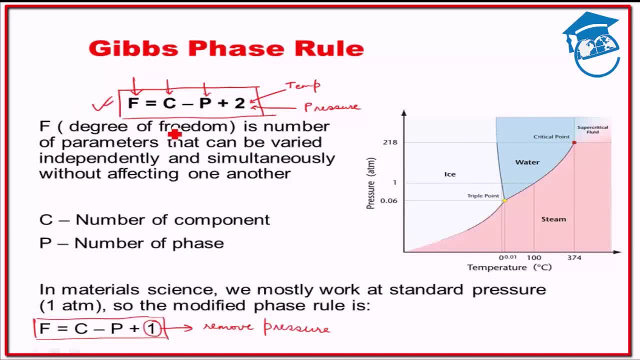 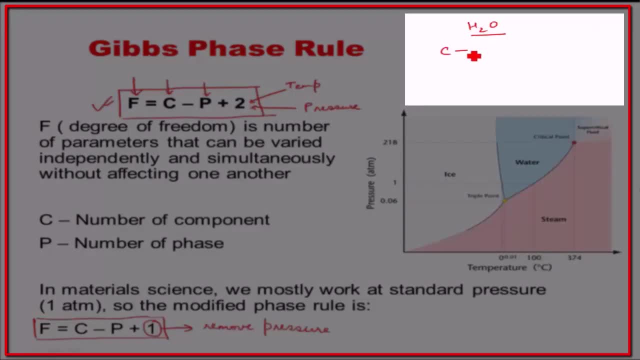 Water, the phase diagram of water, where we will vary both the temperature and the pressure. So we'll be using plus two. Let's see what are the possible components for water. case H2O: What is the component? There is only one component, which is the water right. 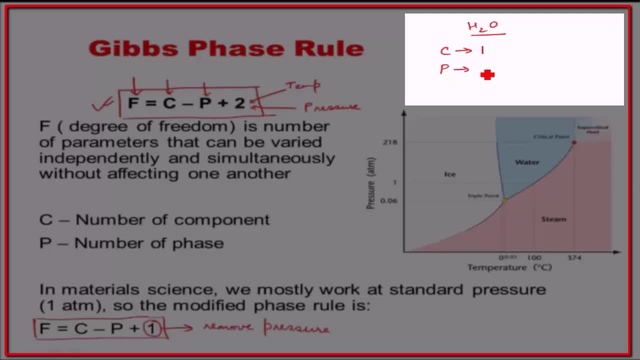 Now, what are the possible phases? The possible phases are: ice water and water And steam. right, These are the three possible phases. Now we need to find, if we need to find out, the degree of freedom at any place we need. 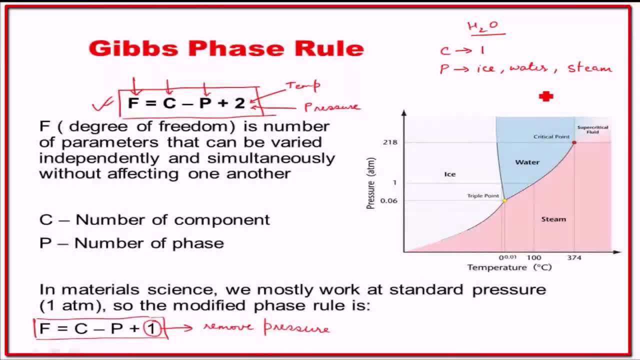 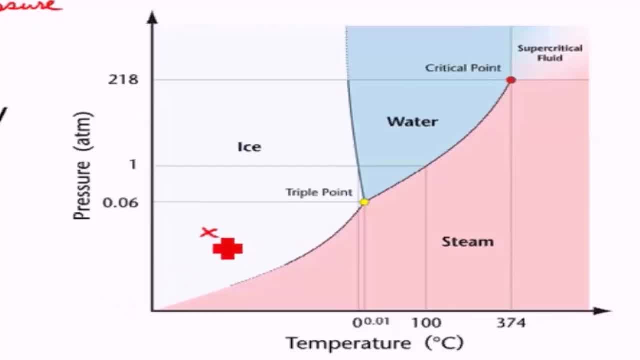 to identify how many phases are there at that place. So to begin with, let's say we want to examine this location. Here the only phase available is ice, right? Since only phase available is ice, we will take P as one, And is already one fixed for all the phase diagram. 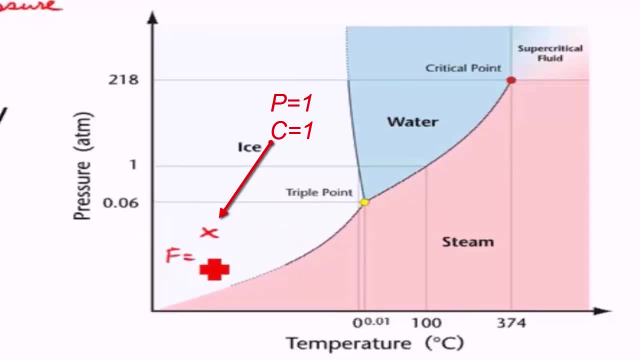 Therefore, degree of freedom over here, F, if we calculate, comes out to be one minus one plus two, which is two. Now, when I say two is the degree of freedom at this location. what does this mean? This means that I can independently vary temperature and pressure here at this location, and still. 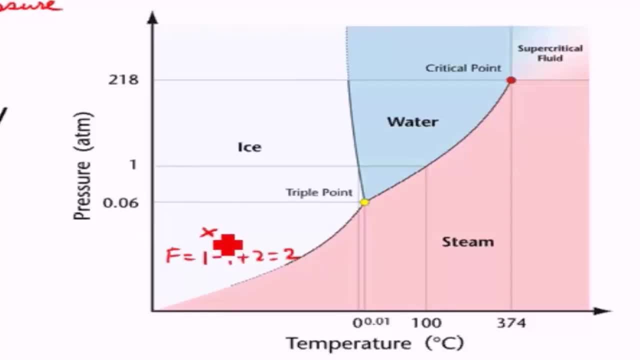 remain in the ice phase itself. Let's say, I increase temperature by this much and increase pressure by this much, I raise this new location, But still we are at the ice phase. okay, A point to note that when you change the temperature and pressure it, these are infinitesimally. 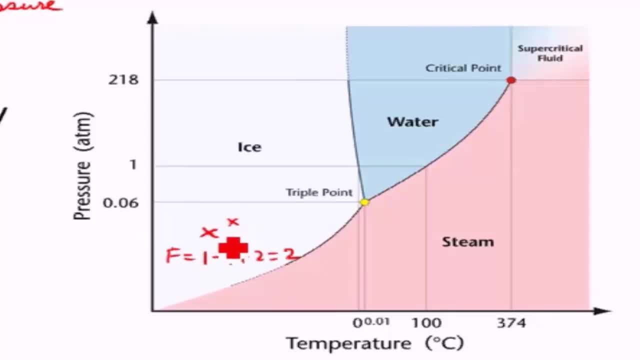 small changes Here I have done just to exaggerate the change. but a degree of freedom means that there will be at least one combination, Combination of change of temperature and pressure which will again give the same phase or phases. Okay, So this means temperature and pressure. both can be changed independently. 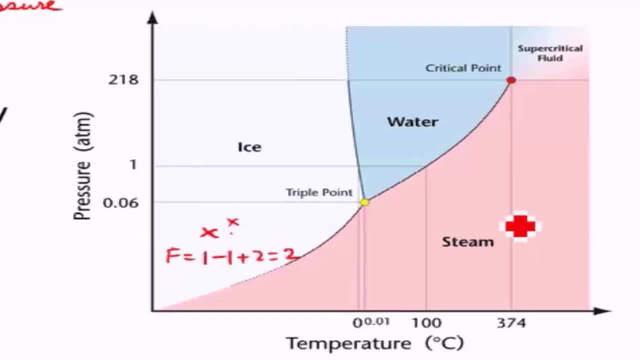 Thereby we have two degree of freedom at this location. Similarly, if we take any steam location we go, change temperature, change pressure. two degree of freedom Similarly in over here, in the water region too. But now just imagine You are at the interface of ice and water over here. 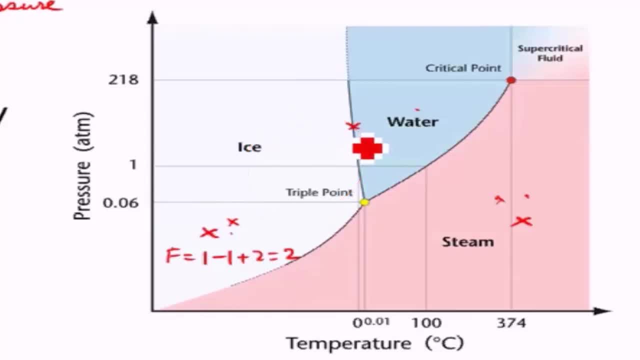 What is happening now? Now, what is happening is you have co-existing ice and water at this location. Thereby, the number of phases no longer is one. For this location, the number of phases turns out to be two. Therefore, degree of freedom is one minus two plus two, which gives me one, one degree of. 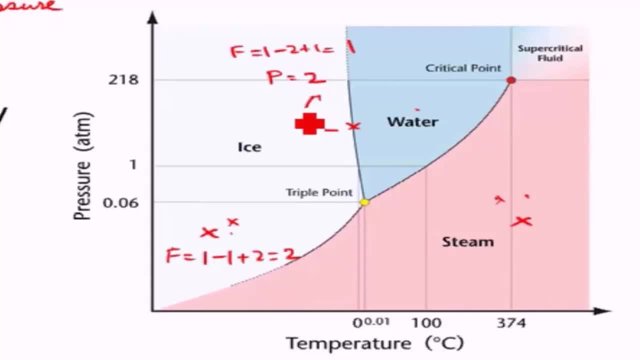 freedom. What does this mean? This means that Temperature and pressure cannot be varied independent of each other to remain at the two phase region. The two phase region is basically this line. So if we change the temperature, if we change the temperature from here till here, then 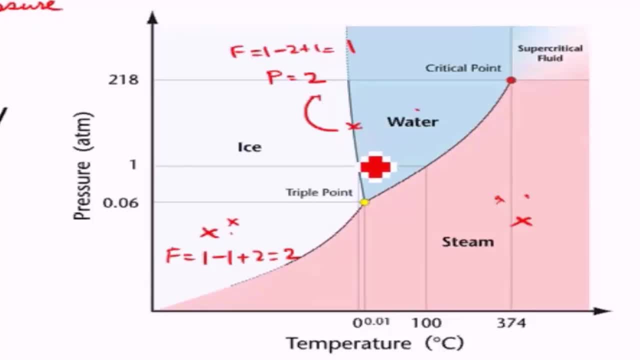 there is only one possibility of pressure, That is, the pressure should come down till here for the system to remain in the two phase region. Therefore, There is only one independent variable right. If we change the pressure from here till here, then the temperature needs to be reduced till. 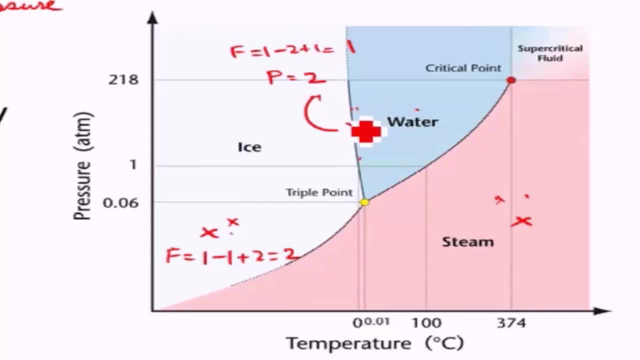 here There is only one possible combination of temperature and pressure. You see that. So the degree of freedom basically says that there is only one possibility, one independent variable, to remain in the dual phase line. Similarly, over here, if I change the pressure from here till here, then the temperature 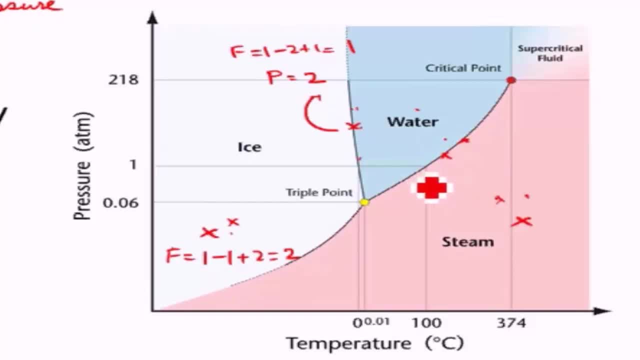 must be changed from here till here. That is the only possibility to still remain in the dual phase line. Okay, In addition to the dual phase line, we have what is known as the triple point. Now let us check out at the triple point. what is the degree of freedom? 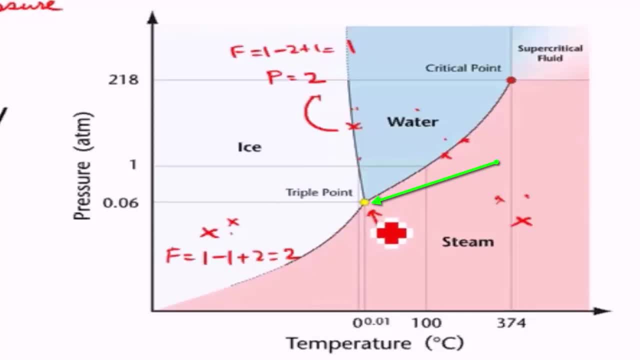 At the triple point. the phases that exist coexist are ice, water and steam. All the three phases coexist. Therefore The P- The number of phases over here, Is Three. It's not two, It's three. All the three phases coexist. 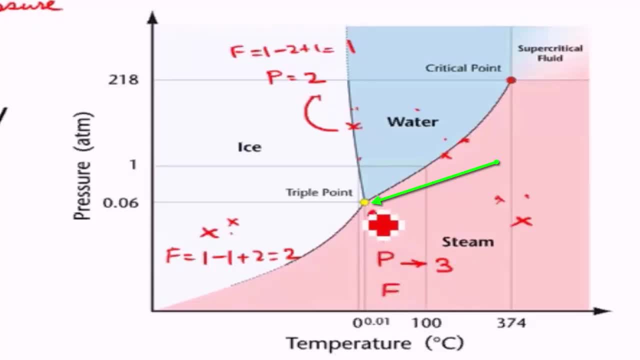 Therefore, the number of degree of freedom for the triple point will be equal to number of components, is one. That is, H2O minus number of phase is three plus two. That gives me zero degrees of freedom. What does this mean? This means that I cannot independently vary either temperature or pressure. 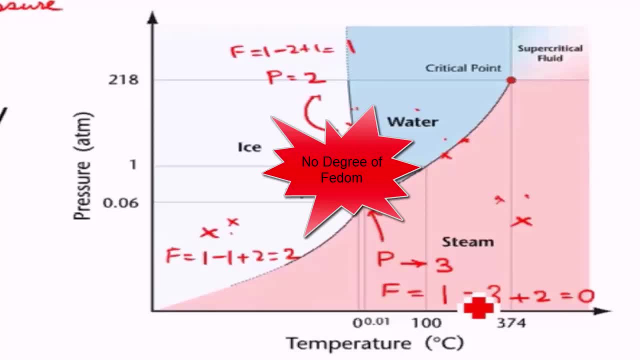 There is no degree of freedom at all. The other way to put this is that triple point is a singular point. It's an invariant point. It's an invariant point. This is only possible at this particular point. There is no alternative point. 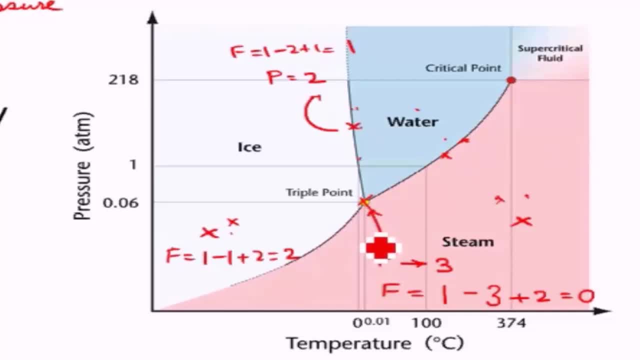 So, if you remember, recall back the eutectic reaction, the eutectoid reaction, the peritectic reaction, Those were invariant points. They were possible only at a given temperature and composition. Here we are dealing with temperature and pressure. 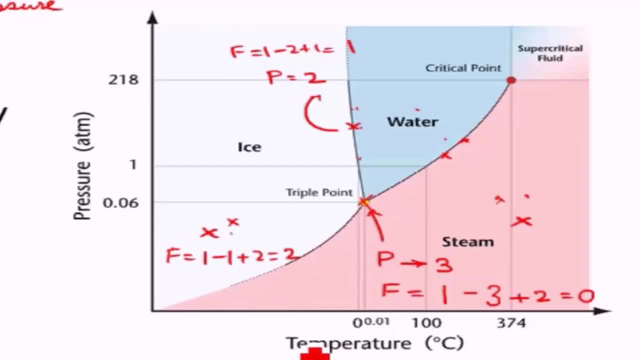 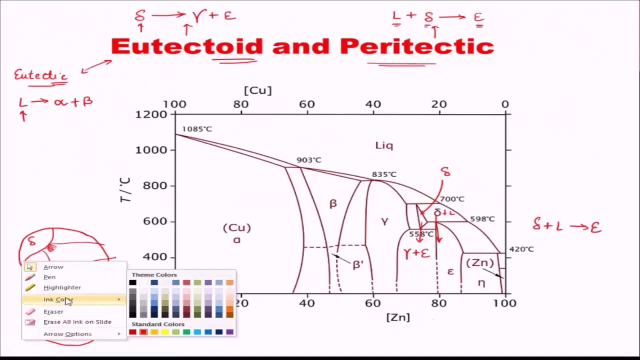 Over there needed to deal with temperature and composition Over there. let me jump back actually Over here. let's see degree of freedom in this case. At this location We have the phases are delta, gamma and epsilon, So we have all the three phases coexisting at this point. 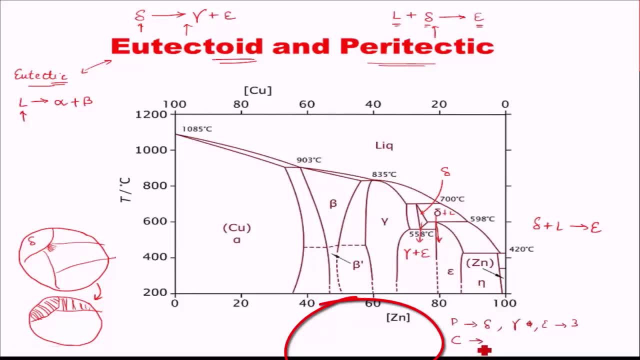 The components we have are two. here, In water, we had one component, which was H2O. Here we have zinc and copper. So we have two components, But since we are in the solid state regime, We are keeping the pressure. We are keeping the pressure constant. 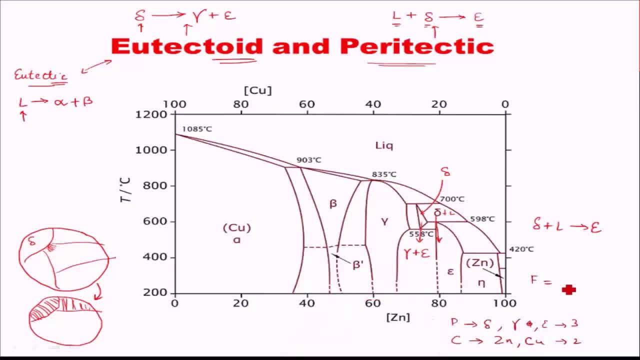 Therefore, degree of freedom can be found out to be C minus P, C minus P plus 1, because pressure is constant. This gives C is 2 minus 3 plus 1 is equal to 0.. So we see again here using the Gibbs rule. 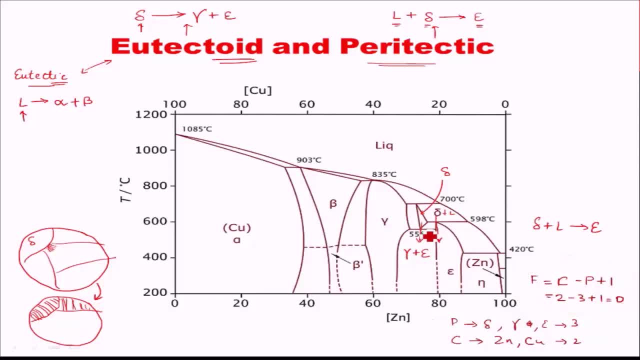 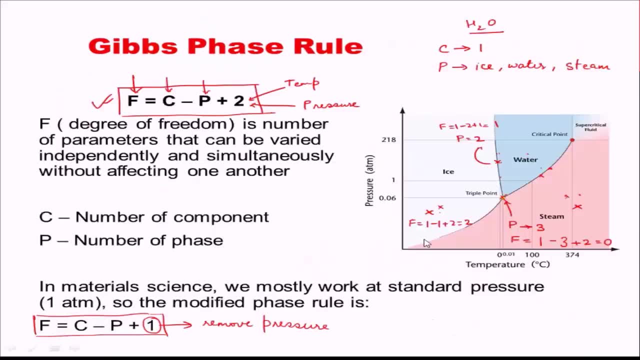 That is, at this invariant point Also, we have degree of freedom 0. Which it should have Because it is a singular point, Like the triple point of water. Okay, So this kind of gives you a rough idea about what Gibbs phase rule is. 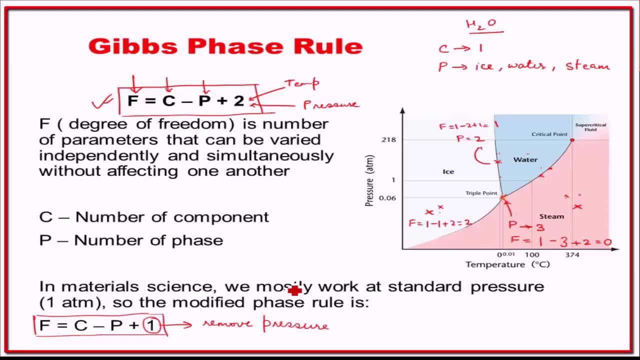 And how, using the Gibbs phase rule, we can engineer the different combinations of temperature and pressure. We can play around And we can, We can, We can decide what temperature and pressure or what temperature and composition we need to take or which are available for a process to have the given phases that we require. 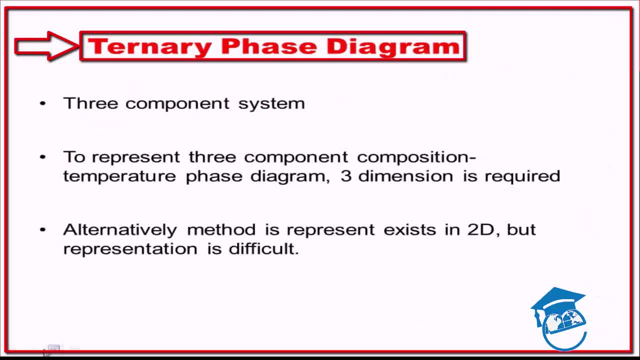 Fine, Now I will briefly talk about ternary phase diagram. Till now, what we have done is we have been talking about binary phase diagram. Binary phase diagram had two components: Ternary phase diagram. Ternary phase diagram has three components. 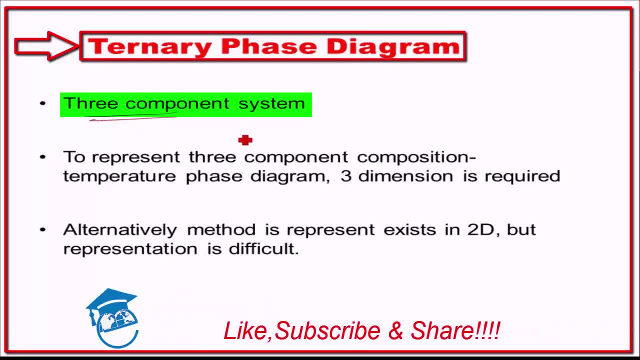 They are three component systems. Now, since there are three components and another variable, the fourth variable will be temperature, Right? So in order to represent it in a phase diagram, you need three dimensions. Therefore, ternary phase diagram are quite difficult to make. 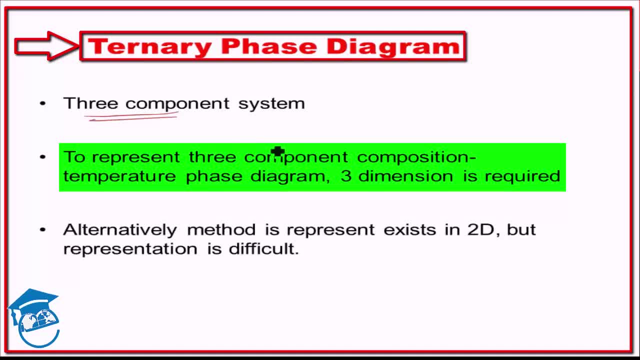 Alternatively, there are methods which can be used to make a ternary phase diagram, For example, For example. Alternatively, there are methods to represent a ternary phase diagram in two dimension also, But you can imagine when you are trying to shrink three dimension into two dimension. 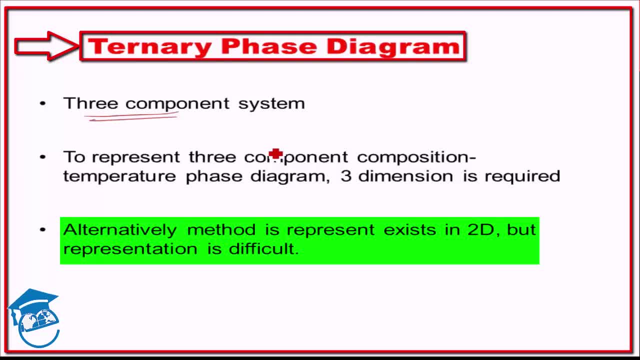